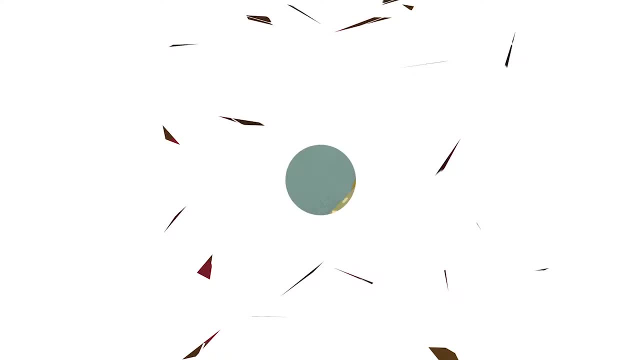 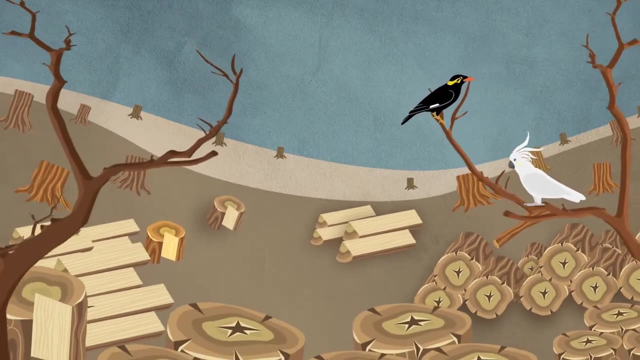 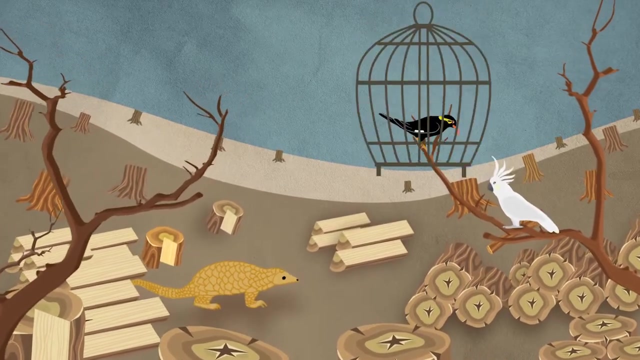 Destructive practices like overfishing, dynamite and cyanide fishing deplete our food supply. Irresponsible conversion of forest land and timber poaching endanger our water supply and leave us more vulnerable to landslide and flooding And pangolins. 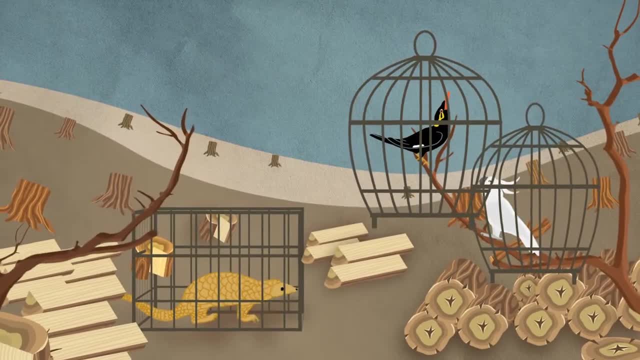 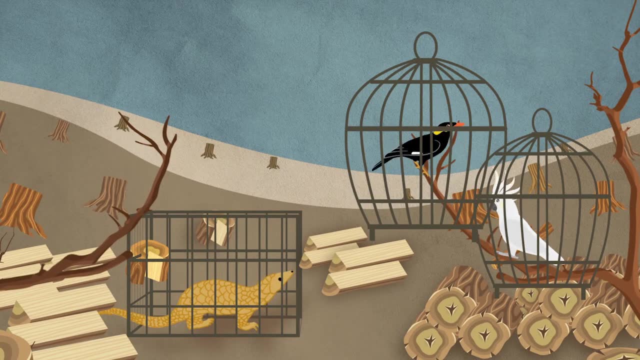 the most illegally traded animal in the world, are being hunted to extinction, not to be killed. That's why we're in danger of losing that connection- Not to mention all the other wildlife being taken from their habitats to fuel the illegal wildlife trade- With our life-saving and life-enhancing connection. 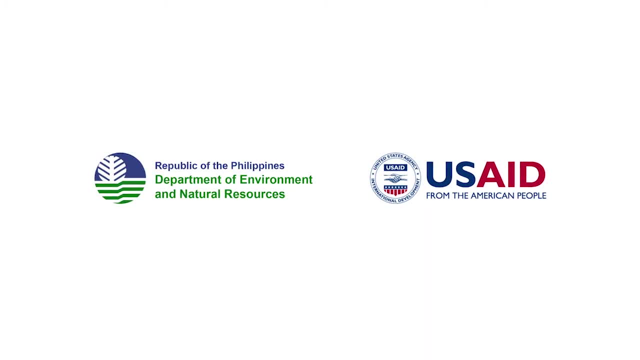 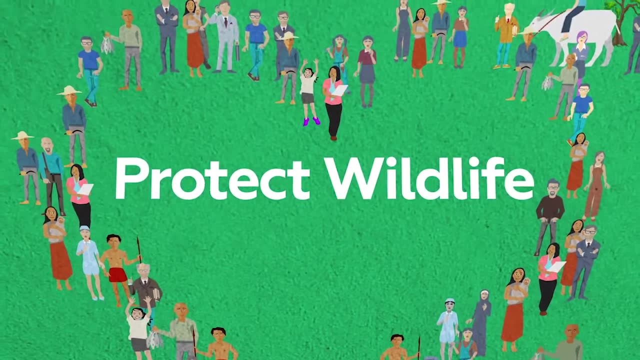 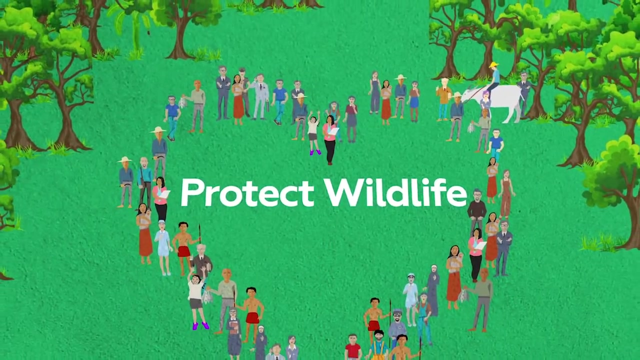 already at risk. USAID and DENR are working with partners to set things right through: Protect Wildlife. Protect Wildlife will partner with communities, governments, universities, enforcers, the private sector and other organizations to make sure our connection to the wild. 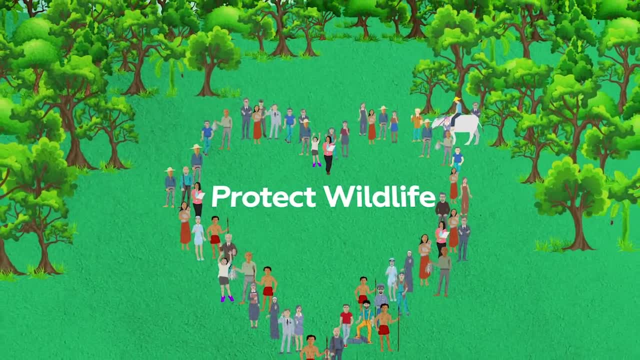 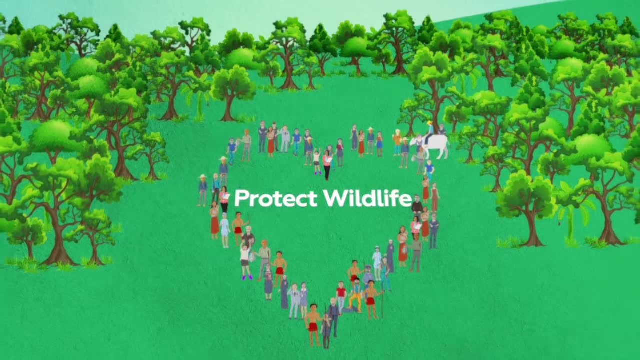 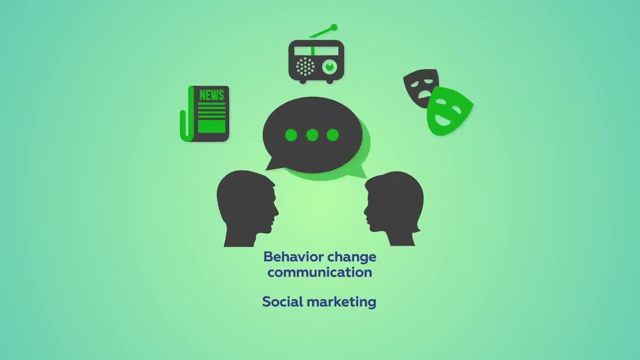 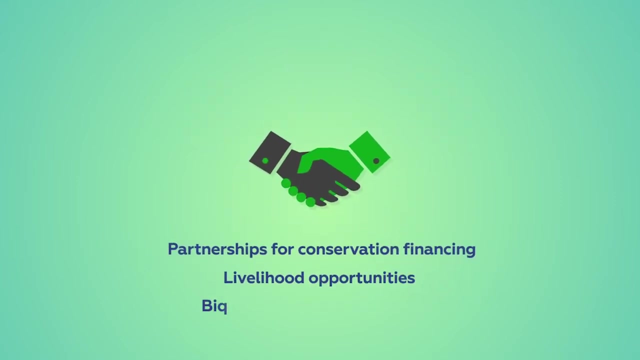 continues to thrive. That means you continue to enjoy all the benefits of nature and wildlife without hurting the very source of these benefits. Protect Wildlife has 5 strategies to make this happen. Use behavior change, communication and social marketing to change people's hearts, minds and actions. Intensify public and private partnerships. 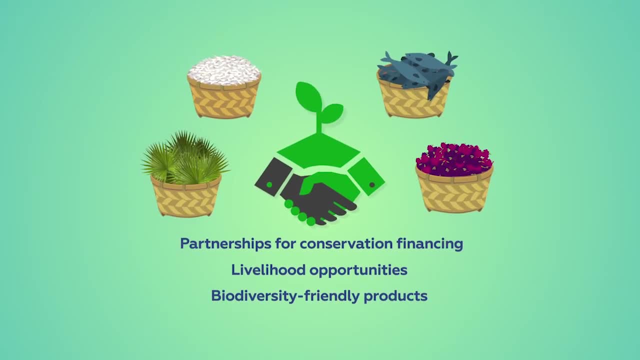 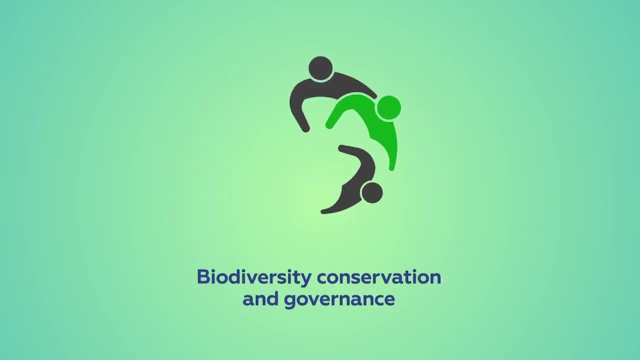 that can fund conservation activities and create livelihood opportunities through biodiversity friendly products. improve the ability of local government and civil society to create policies and plans so they can drive the process of conserving wildlife and natural resources under their care, ensuring their community grows sustainably. work with universities to undertake research. 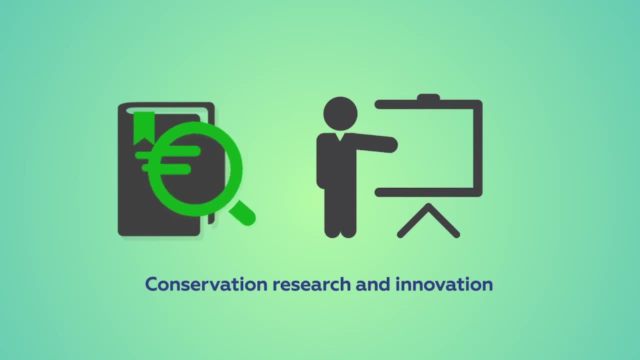 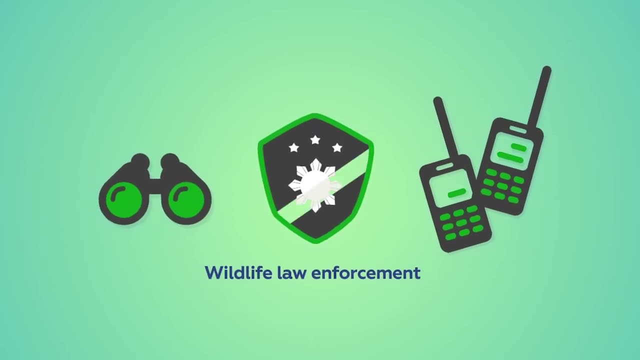 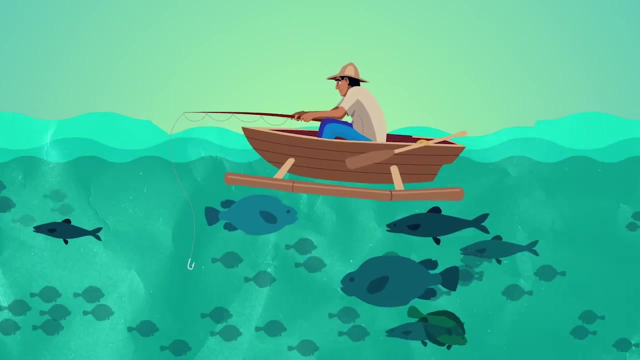 and develop technologies that aid conservation and train enforcers to better enact and follow through on wildlife law enforcement to decrease illegal and destructive activities. When we fish at the right time at the right place using the right gear, fish stocks will boom When we use our lands. 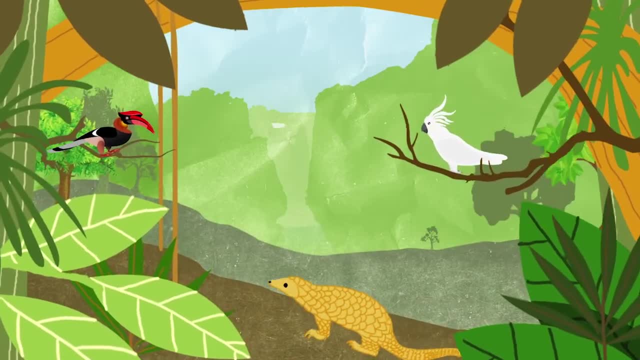 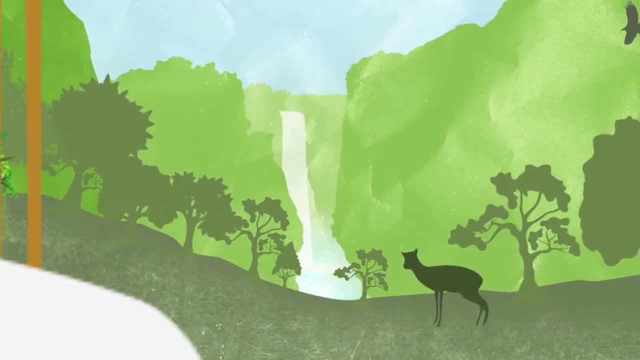 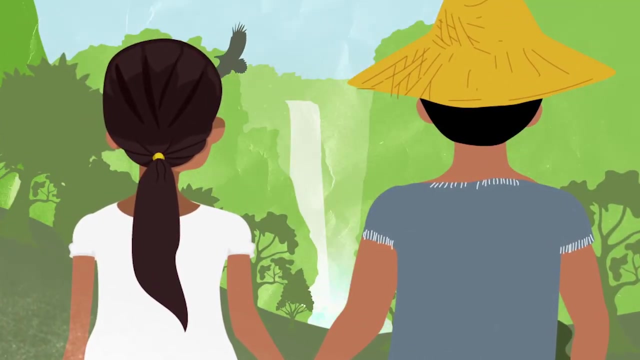 responsibly. there will be a solid supply of clean water. When habitats are protected, important species flourish, and it all comes back to you. You'll enjoy the benefits and experience what it truly means to be connected to the wild, After all. 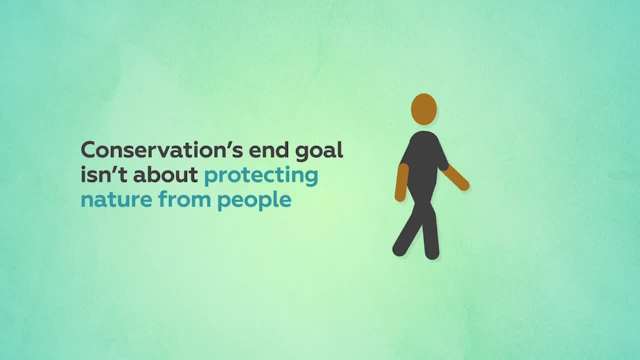 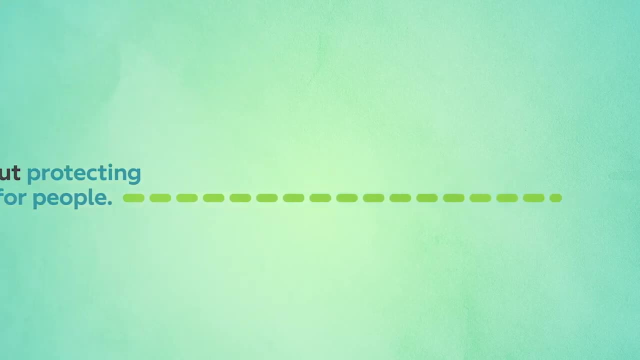 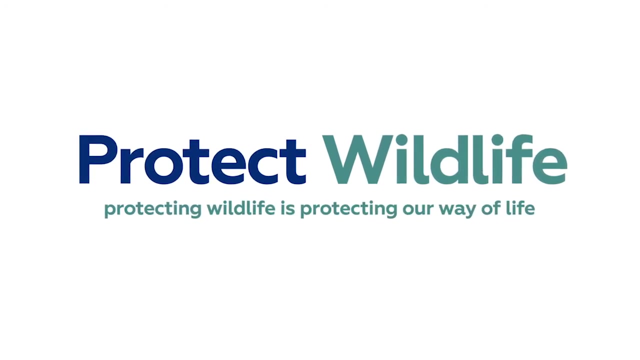 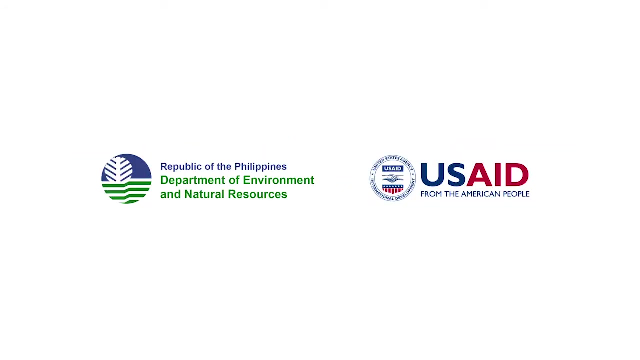 conservation's end goal isn't about protecting nature from people. it's about protecting nature for people. Let's make sure we keep that connection going. Protect wildlife. Protecting wildlife is protecting our way of life. Thank you for watching Fart Parent%. Fart B assets Fart: Parent% Fart. 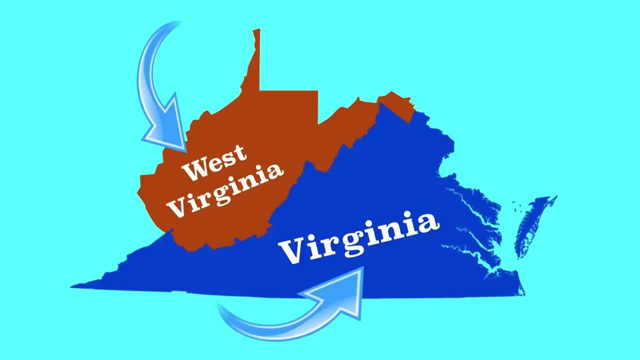 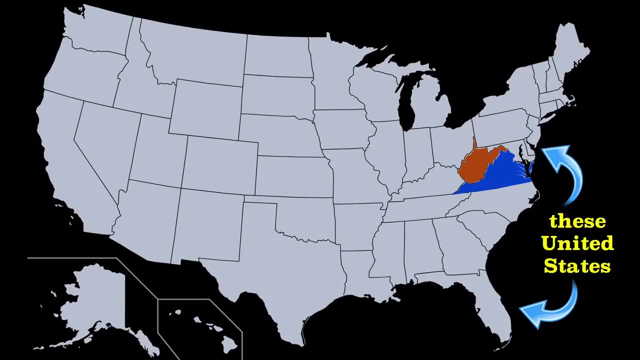 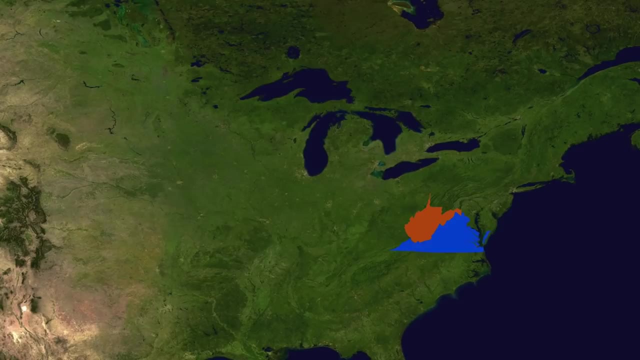 Virginia and West Virginia, or the Old Dominion and the Mountain State, Two bordering southeastern states in these United States. that, uh, used to be one state. Yeah, let's go ahead and dig into some history and look at why that is. Humans have lived in the modern-day Virginias for. 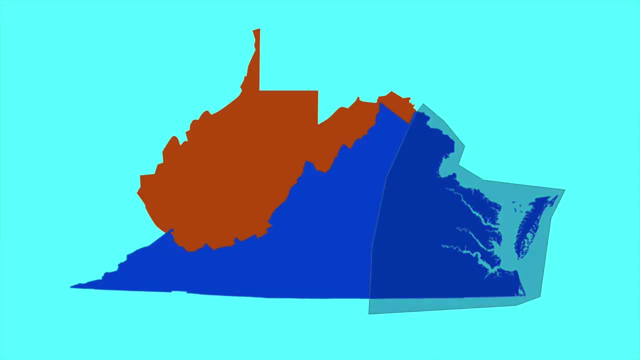 thousands of years Before European arrival, eastern modern-day Virginia was dominated by the Powhatan Confederacy. However, several other American Indian tribes are native to the area, including the Tutelo and Saponi, Catawba and Cherokee Meanwhile modern-day West Virginia. 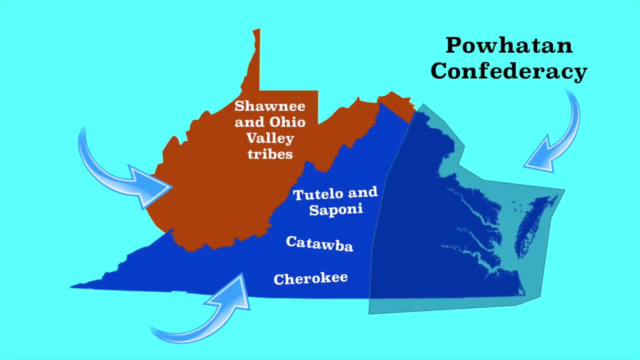 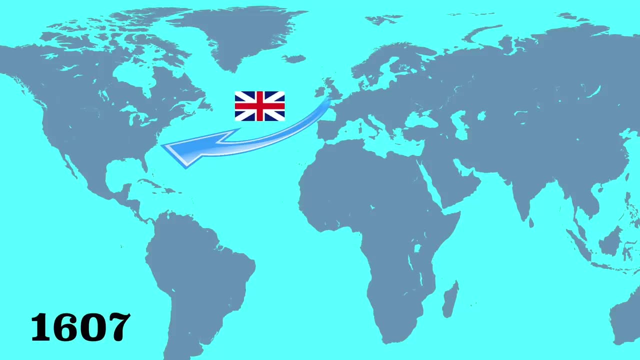 was home to various Shawnee and Ohio Valley tribes, but also the Tutelo and Saponi and Cherokee. In 1607, the English came over. Wait a second. is that why I'm speaking English to you right now? Anyway, the London Company. 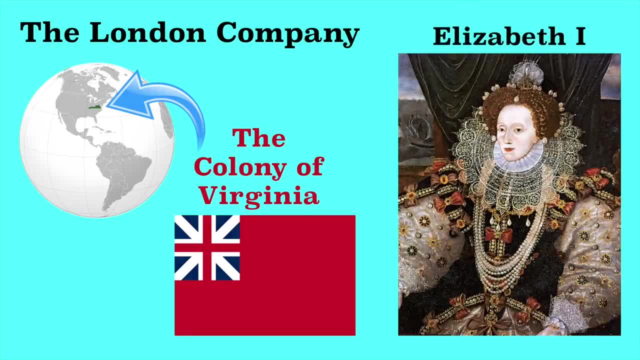 established the Colony of Virginia named after Queen Elizabeth I of England, who was known as the Virgin Queen Get it. The Colony of Virginia was the first permanent English colony in the Americas, which is why Old Dominion is the state nickname today. by the way, 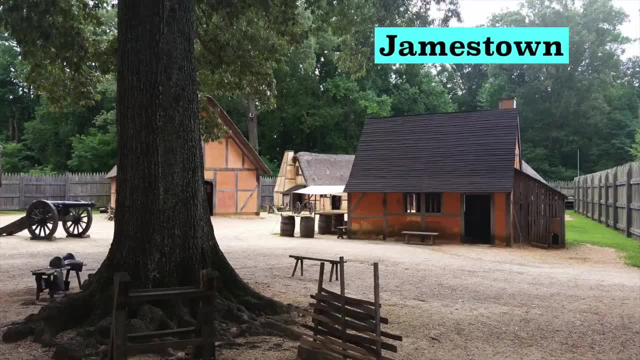 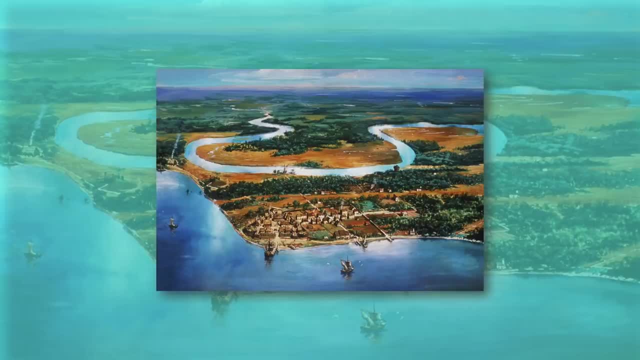 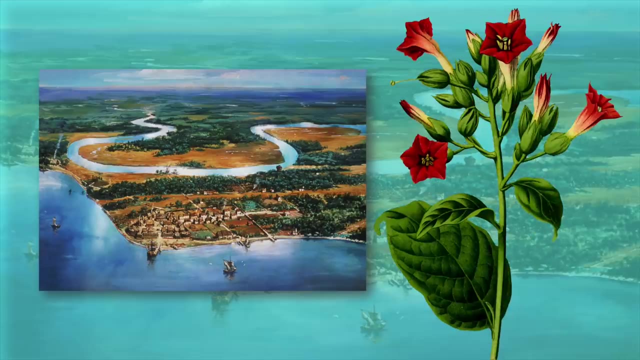 After a rough start, the settlement of Jamestown, located on the north bank of the James River, eventually thrived as the first permanent English settlement in the Americas. They first settled the area for gold, but never found any. No worries, They soon figured out how to grow tobacco, which might as well have been gold since. it became so valuable. That was mostly thanks to this dude, John Rolfe, who also famously made peace with the Powhatan Confederacy by marrying Chief Powhatan's daughter, Pocahontas. There was later a crappy Disney movie about Pocahontas. Anyway, European settlement steadily increased. 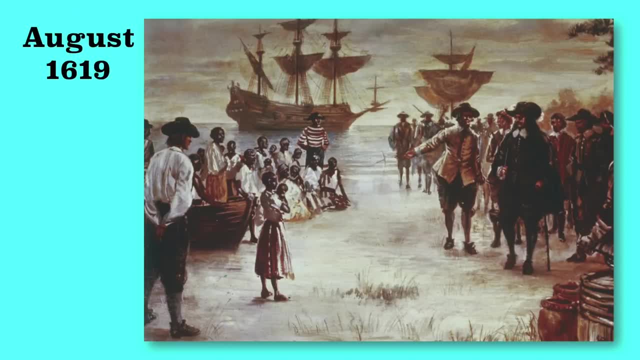 became the Pouhatan Confederacy In August 1690,. the Pouhatan Confederacy. the Pouhatan Confederacy became the Pouhatan Confederacy In August 1690, the first recorded slaves from Africa arrived near Jamestown and worked in tobacco fields. Over the following decades more, and